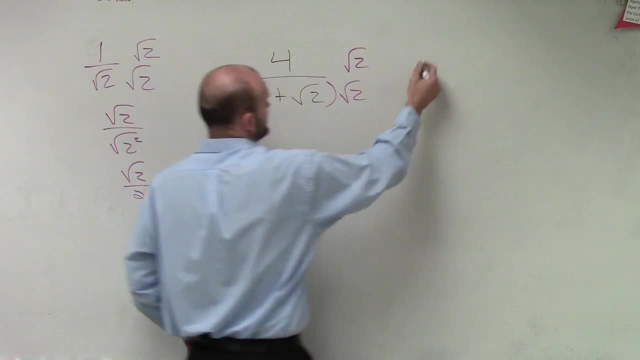 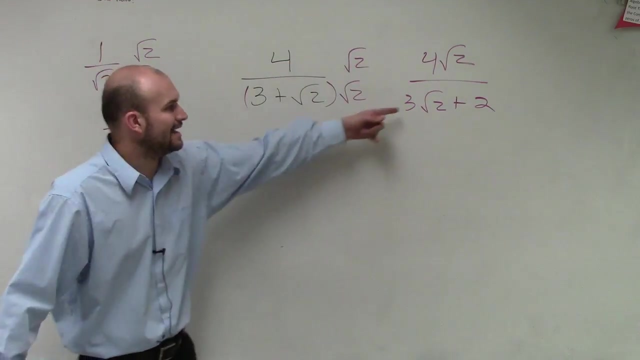 But if you do that here, then you end up getting 4 radical 2 over 3 radical 2 plus 2.. Again, you still have a radical on the bottom right. So you're kind of what we call treading your. 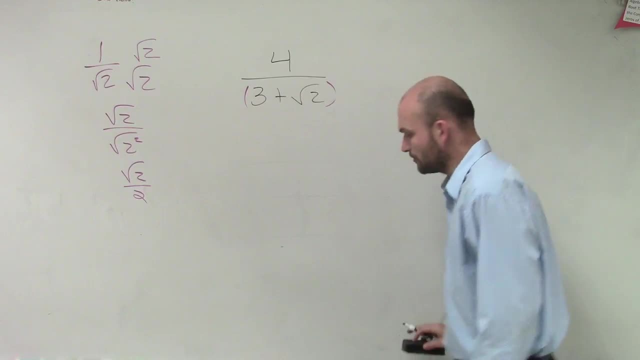 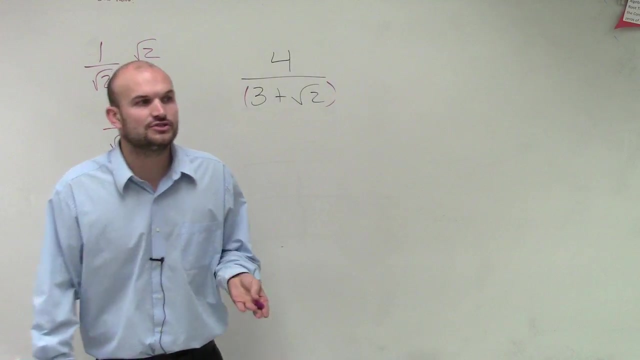 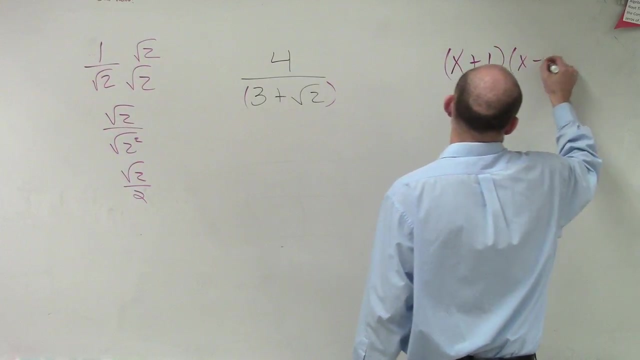 tires in mud, You're not going anywhere. So what we need to do is we need to think of a number that we can multiply by 3 plus the square root of 2. that is going to undo my square root. Now there's a special case, If you guys remember: x plus 1 times x minus 1.. These 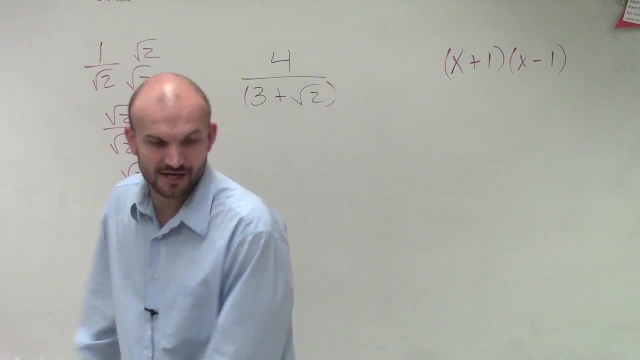 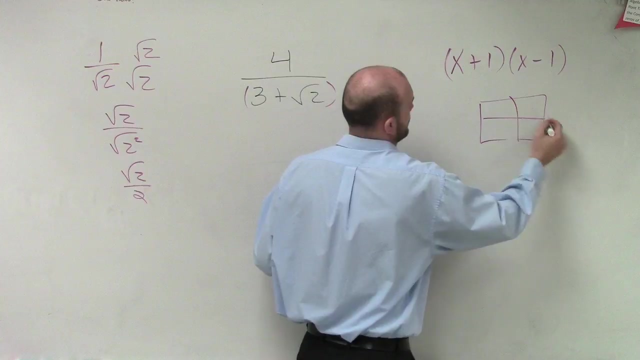 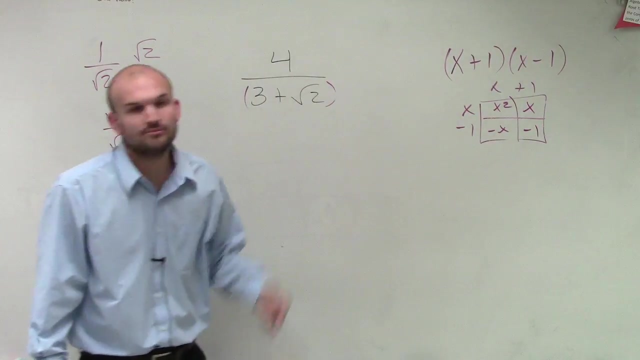 are what we call a difference of two squares, And the important thing about difference of two squares is: remember, when we multiply these out- x plus 1, x minus 1, we get x squared, x negative, x negative 1.. Right, What happens to my middle terms? They add out to 0,. right, They add to 0,. so they're. 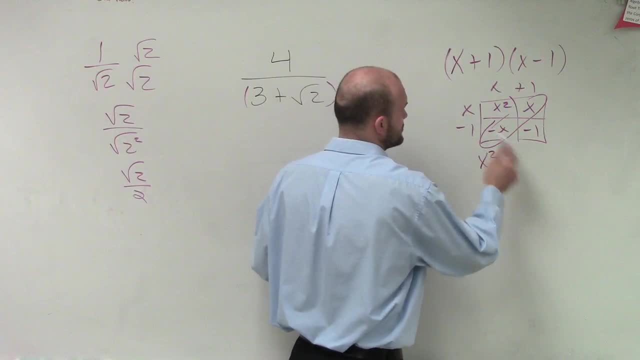 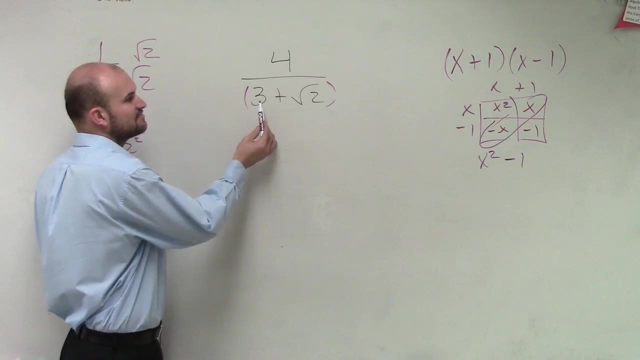 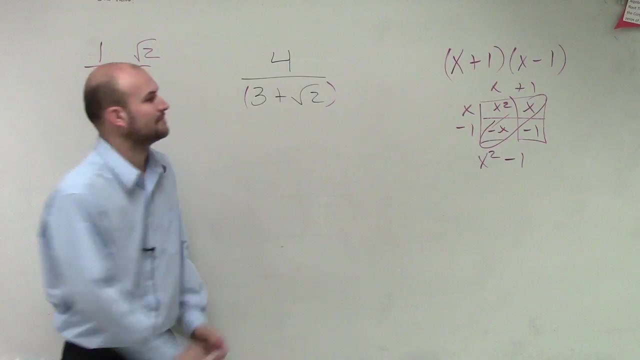 eliminated. So, therefore, what I really just did is added the first two terms and the last two terms. right, Which is pretty cool. Now, ladies and gentlemen, if I just multiplied my first two terms and my last two terms, would I then get rid of my square root? So, 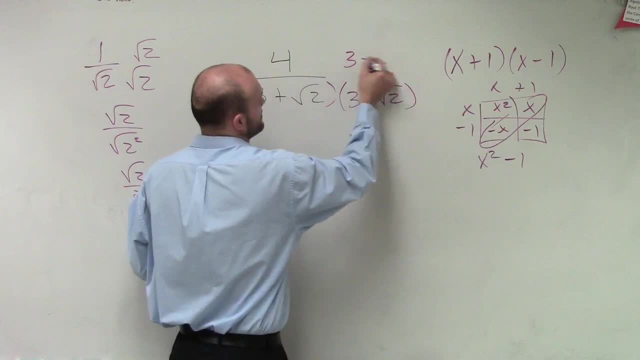 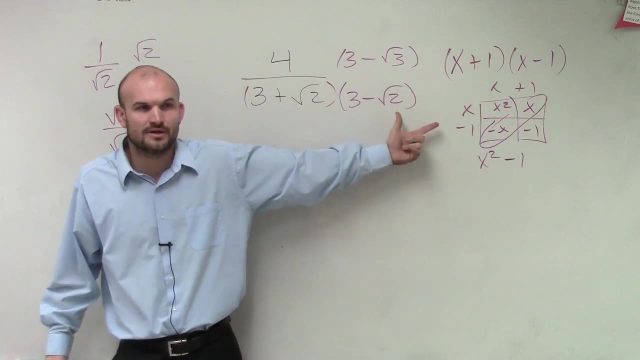 let's multiply by what we call the conjugate, And the reason why we multiply it by the conjugate is: notice: the conjugate is going to create a difference of two squares. So now all I have to do is multiply my first two terms and my last two terms, because then what that's? 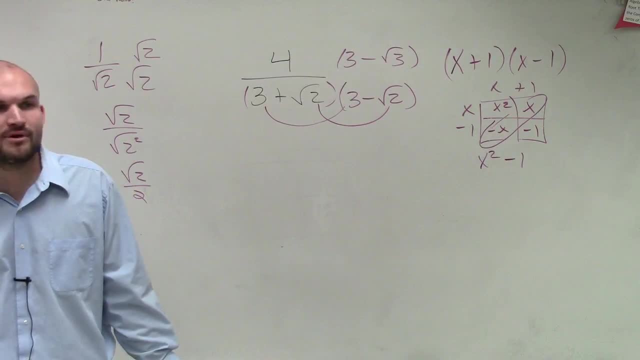 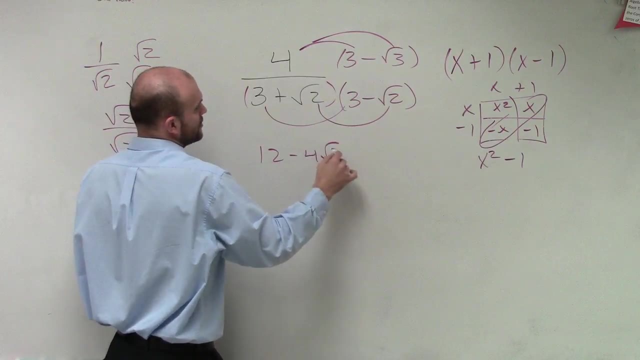 going to do is- I don't have to worry about my middle terms because it's a difference of two squares- So I distribute the top, which I get 12 minus 4, square root of 3.. Then I divide it by 3 times 3 is 9.. Square root of 2 times negative square root of 2 is going: 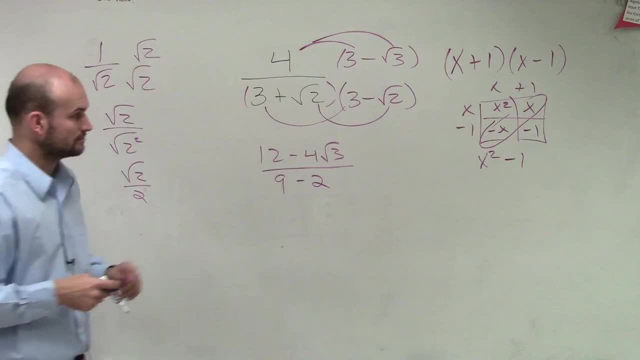 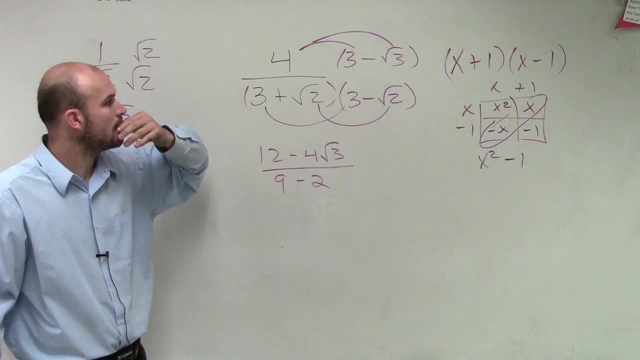 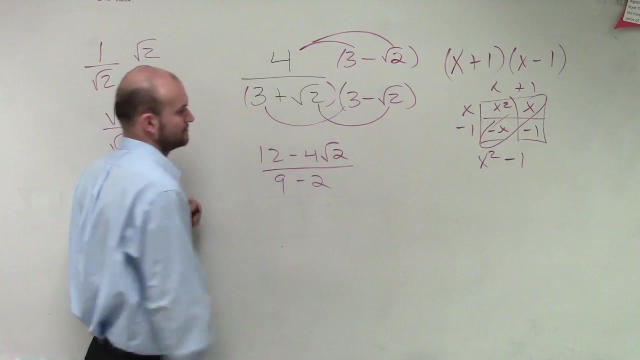 to be a negative. Wait, why'd you put 3 minus square root of 3?? You have to multiply on the top and the denominator, Yeah, but that's the square root of 2 at the bottom. I don't know, I'm like losing it. There you go, Thank you. So does everybody follow me?